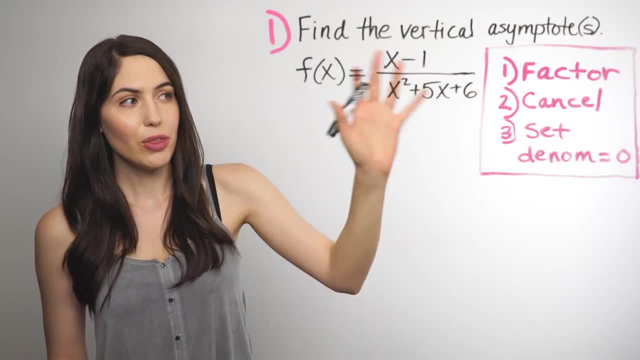 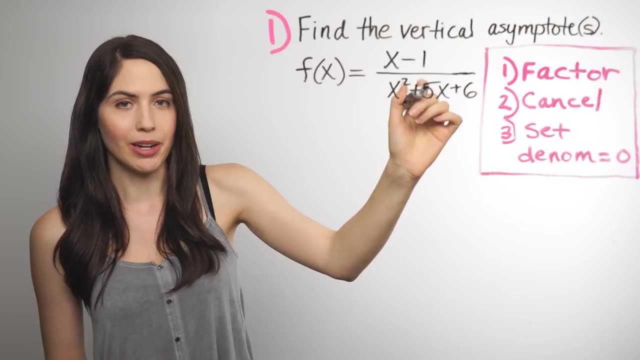 Okay, so here are the three steps you can always use to find the vertical asymptotes of a rational function. The first is to factor the top and bottom, if you can, and all that you can, I'll show you what I mean. 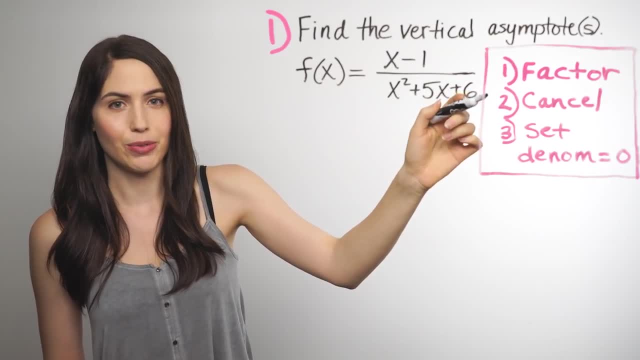 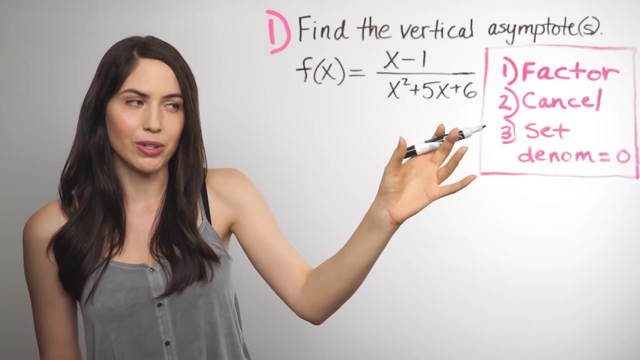 The second is to cancel any common factors from the top and bottom, to simplify. And the last step is to take the bottom, the denominator, and set it equal to zero to find the vertical asymptotes. So let's try it for this function. 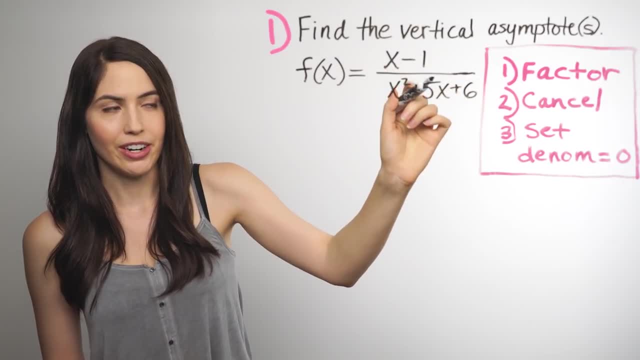 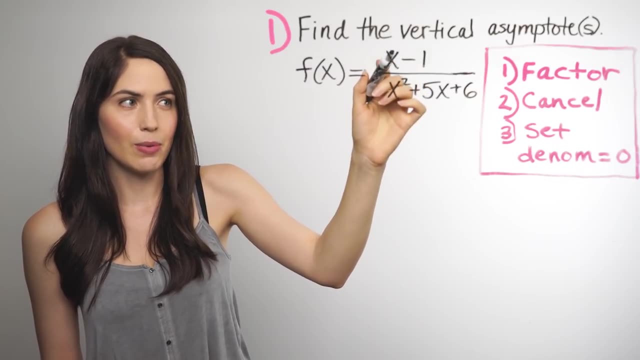 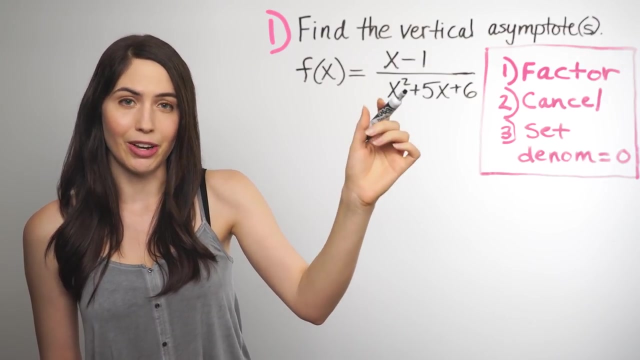 The first step is to factor the numerator and denominator, if you can and all that you can. So you can't factor the top in any way, but the bottom you can factor. It's a quadratic And if you want more help on how to factor quadratics, I have a video for that so you can check that out. 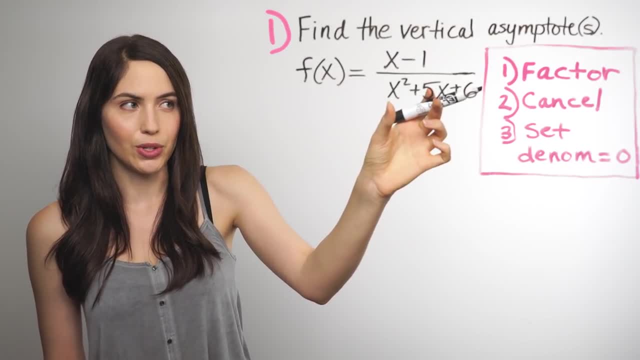 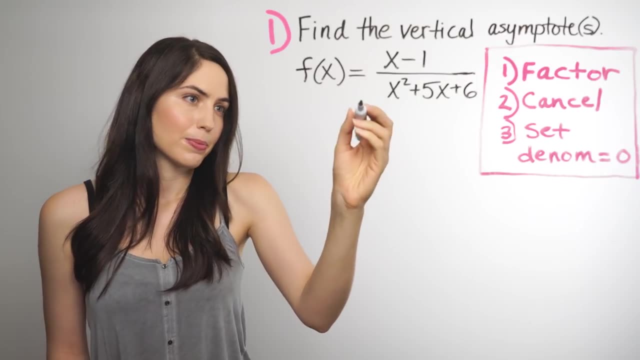 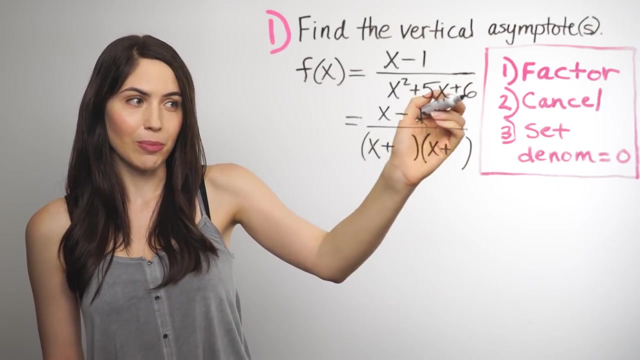 But basically the idea is, you want to break this into two separate factors that start with x, So x plus a number times x plus another number. Okay, and what you want are two numbers here, two numbers here that multiply to 6 and add to 5.. 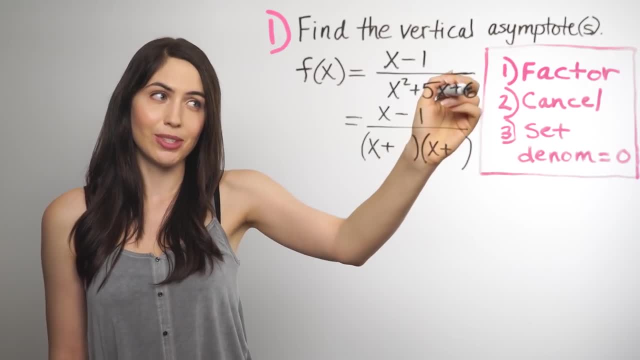 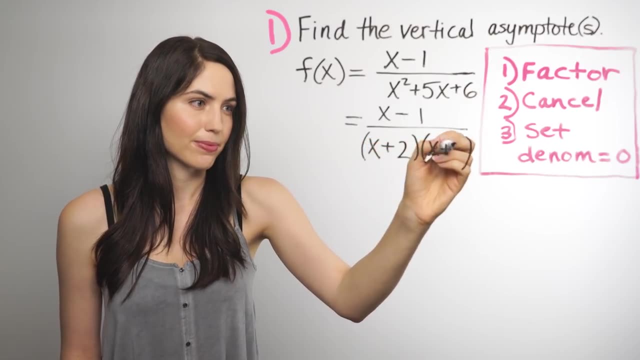 And those two numbers would be 2 and 3, since 2 times 3 is 6, and 2 plus 3 is 5.. So in here we have 2 and 3.. And that's all that you can factor for this rational function. 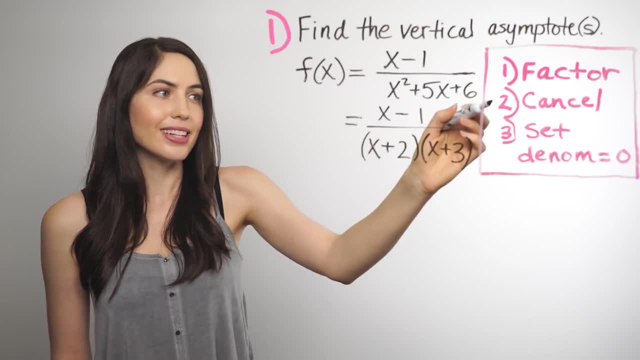 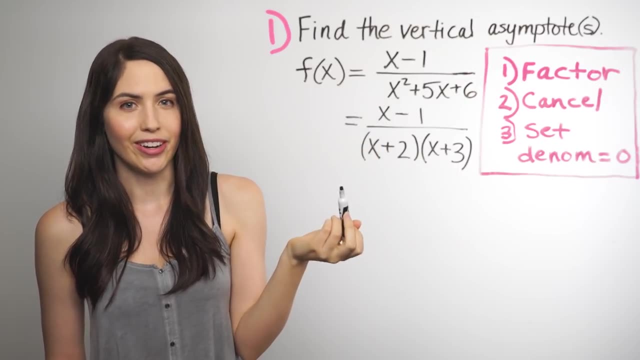 So that's the first step You factored. Second step: see if there are any similar terms on the top and bottom that you can just cancel out. In this example there are not any. The top has different factors from the bottom completely, so you can't do that here in this particular case. 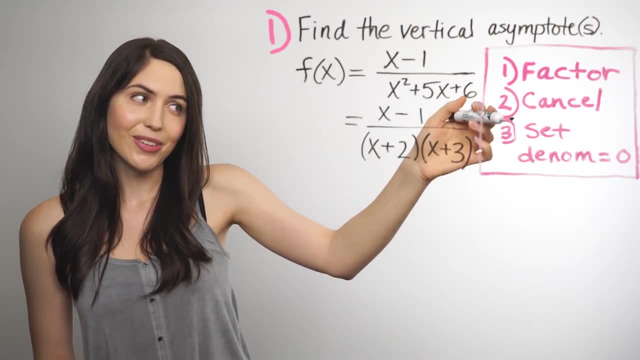 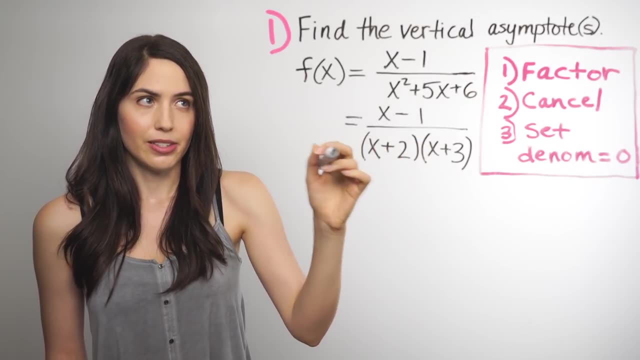 So we move on to the last step, thankfully, which is to take the bottom, the whole denominator, and set it equal to zero And solve for the real zeros of the denominator. So take the whole bottom and set it equal to zero. 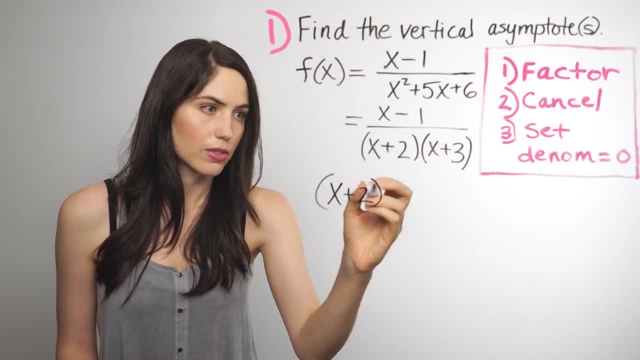 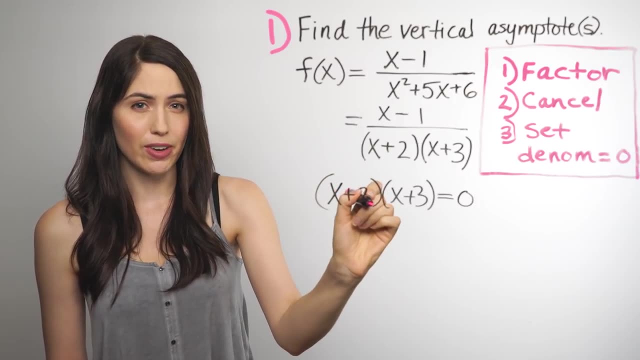 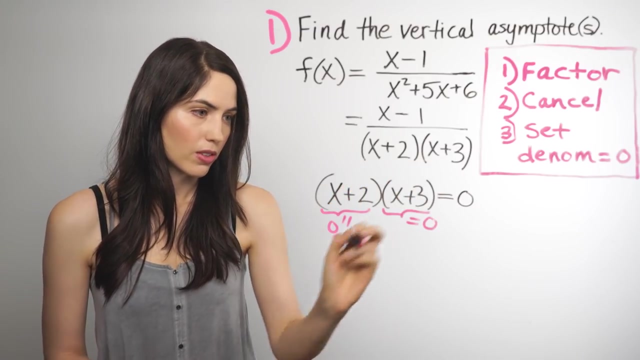 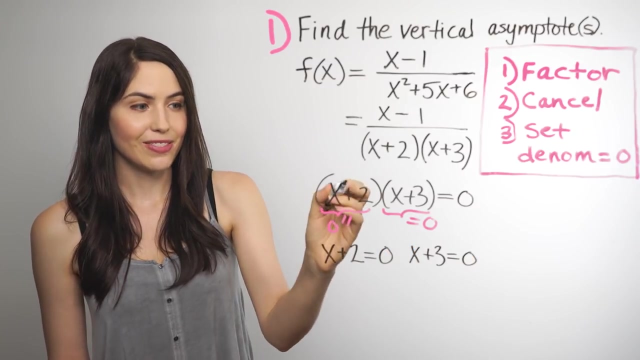 And to solve something like this- you may already know this, but you have to take each factor separately and set each of these equal to zero individually. So take each of these and set them equal to zero And solve for x. Get x alone. 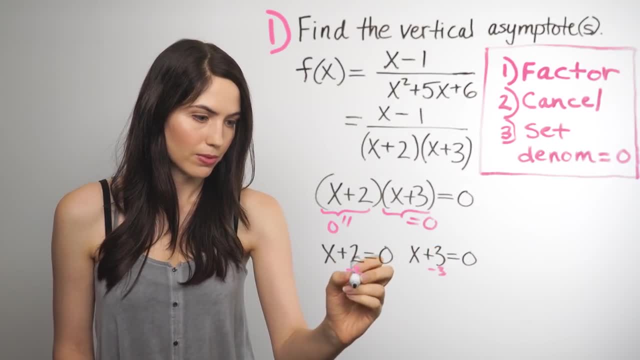 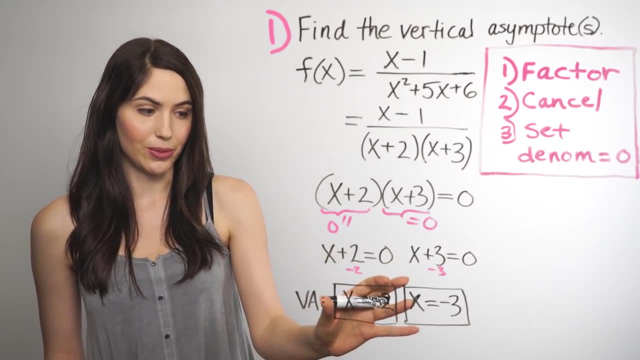 Sum the integral of x. So x equals negative 2 here and x equals negative 3 there, And just go ahead and add x here. So these are your vertical asymptotes. If you solve for x in each case, get x alone. 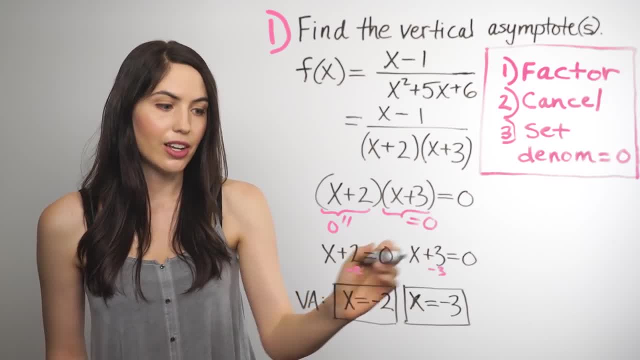 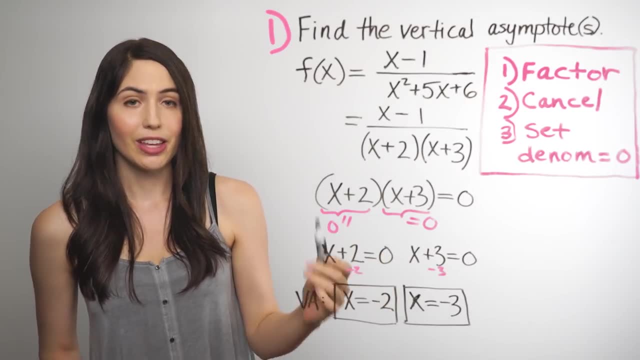 Subtract a 2 here, subtract a 3 there. You have x equals negative 2 and x equals negative 3.. These are your answers. The vertical asymptotes, if you have any, will always be at: x equals some number or numbers. 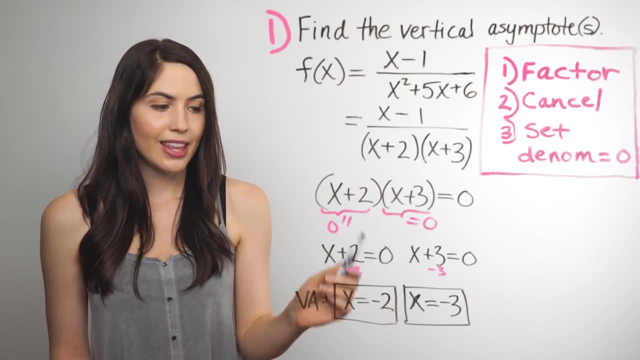 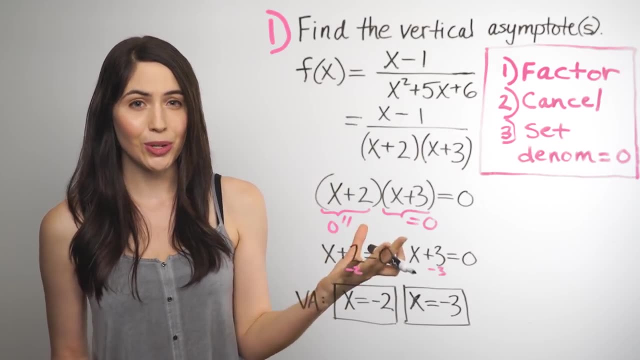 These are your vertical asymptotes, If you have any, will always be at: x equals some number or numbers, numbers, and they correspond to invisible vertical lines on the graph. so this is your answer. you don't need to do anything more, but I want to show you. 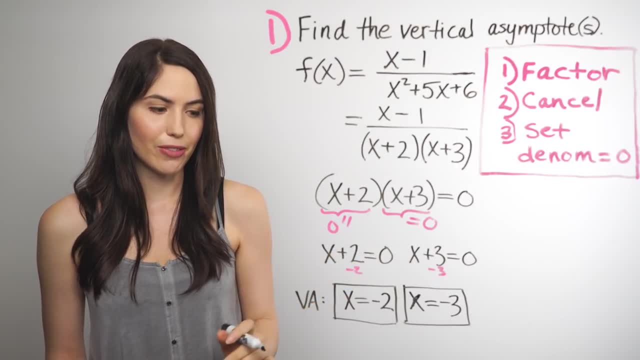 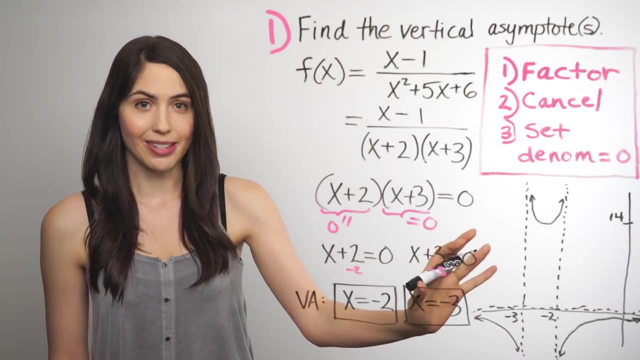 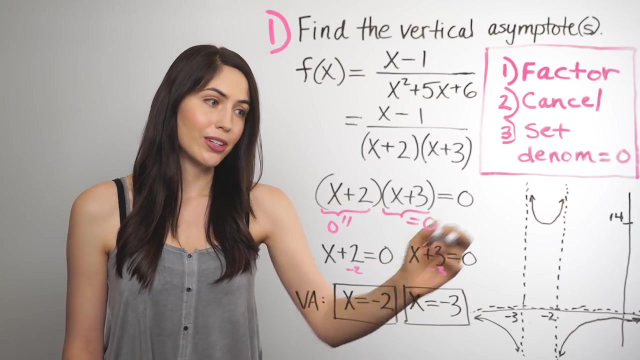 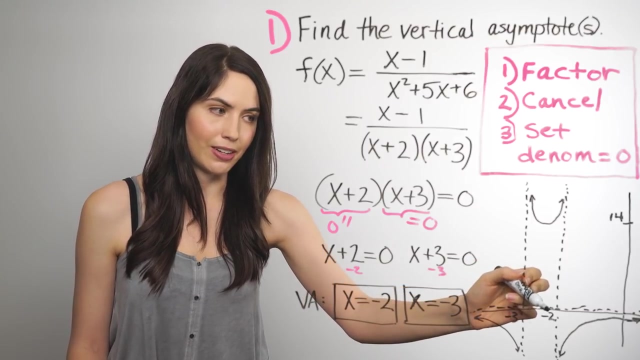 what this means. so let me show you that on a graph. okay, so again you don't have to graph this, but just so you know what the vertical has into its mean. these answers- x equals negative 2 and negative 3- correspond to dotted invisible lines, vertical lines on your graph at: x equals negative 3 and x equals negative. 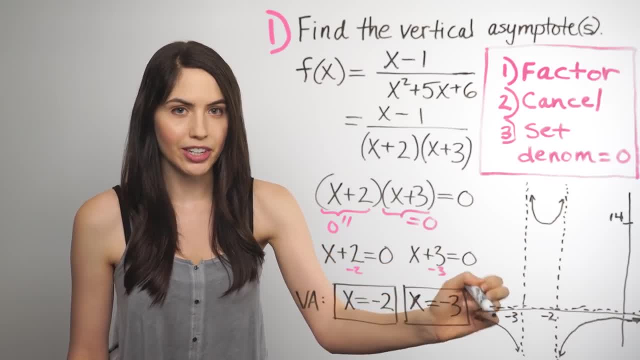 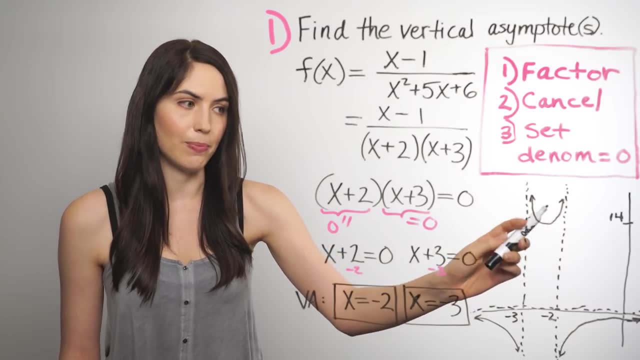 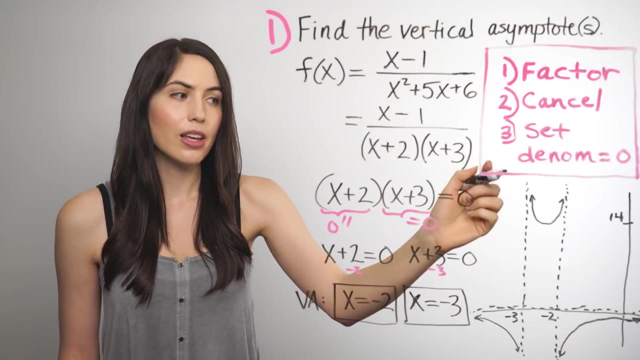 2 and your curve or your graph will never cross those invisible vertical lines or touch them, reach them. so, like up here and in this branch, each side is shooting toward positive infinity if you go up, but when it does that, it will never go beyond. x equals negative 3 or negative 2 on either side. and for these, 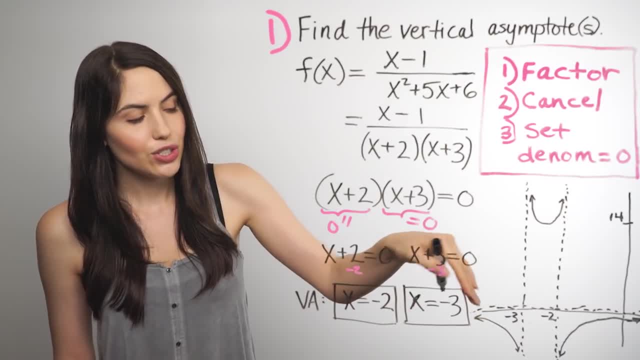 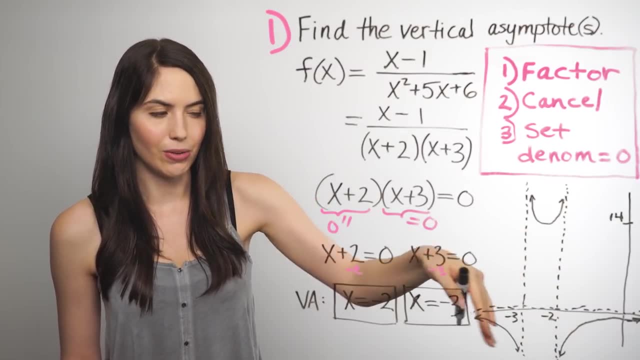 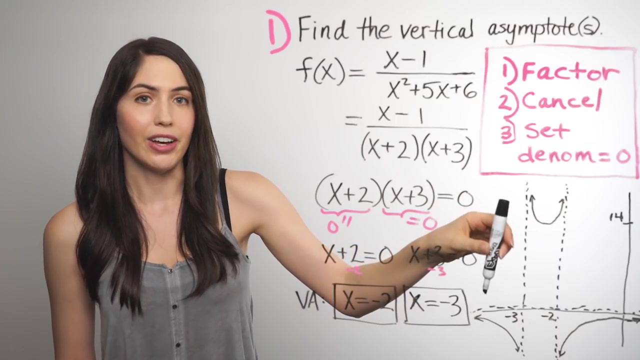 branches down here same idea. they're each shooting down to negative infinity here and here, but they will not cross to the left of negative 2 or the right of negative 3. so those vertical lines are the asymptotes, are where the function is not defined for x. 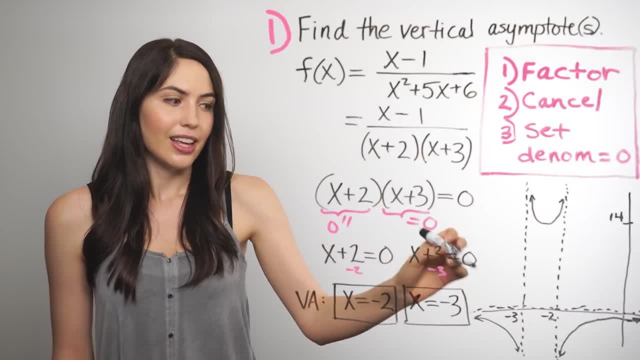 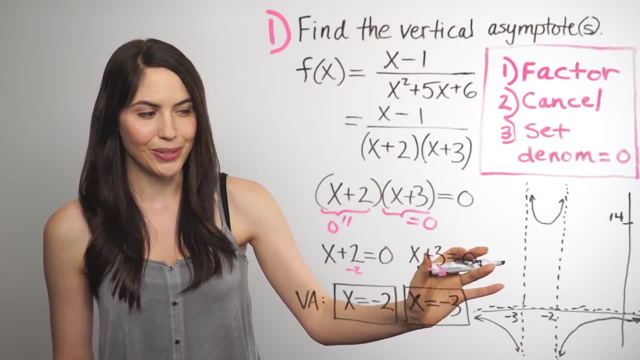 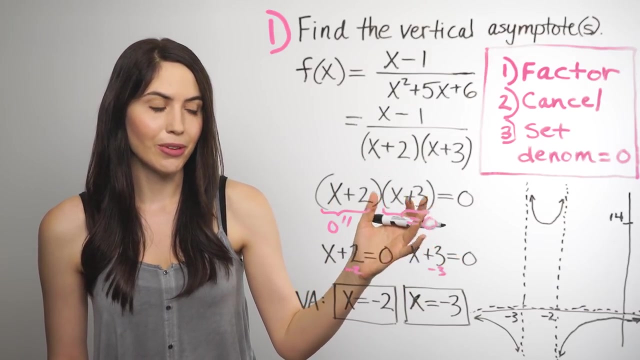 where it does not exist for x- and I know that there's another dotted line on here- this horizontal one at y equals 0. I'm not trying to confuse you. that is a horizontal asymptote, so it's different- and you find it in a different way- from the vertical ones. I 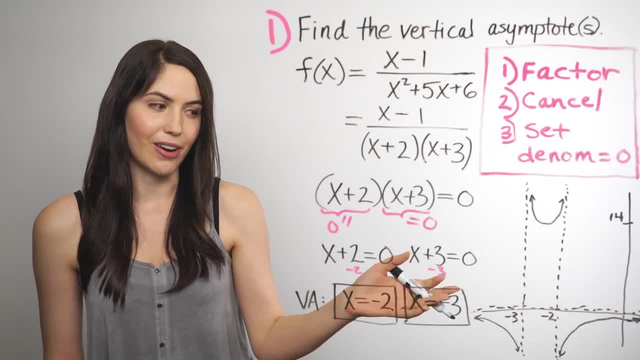 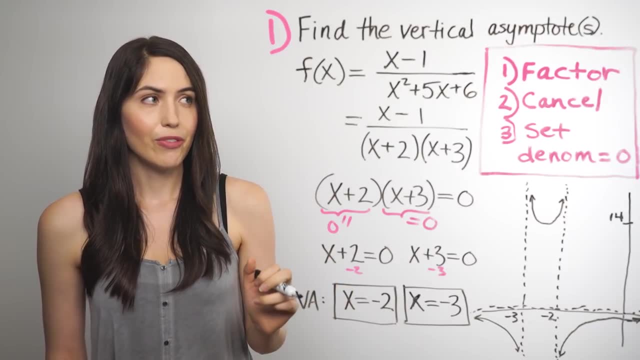 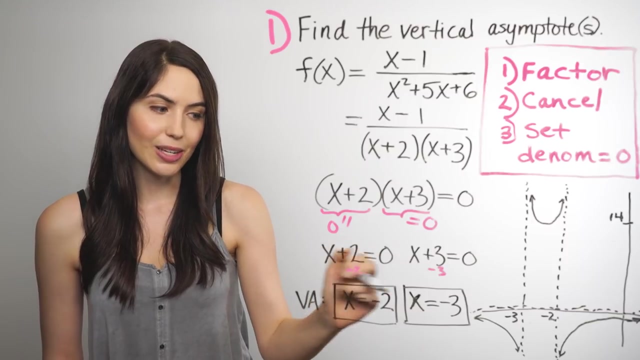 actually have a video on how to find the horizontal asymptote so you can check that out if you want. but basically, in a nutshell, if you want to find the vertical asymptotes, if your function is in its most simplified form, the vertical asymptotes will be at: x equals the real zeros of the denominator at the bottom. 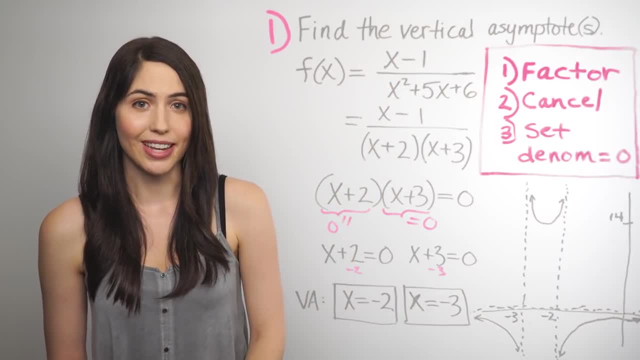 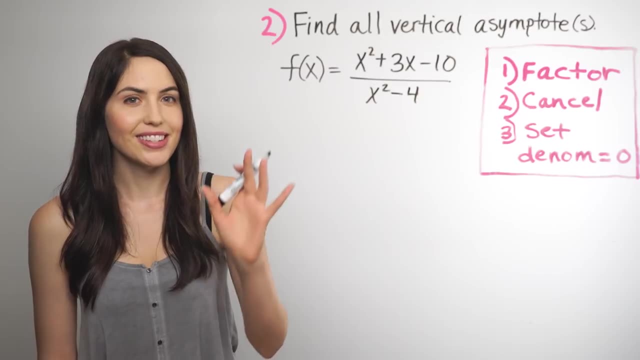 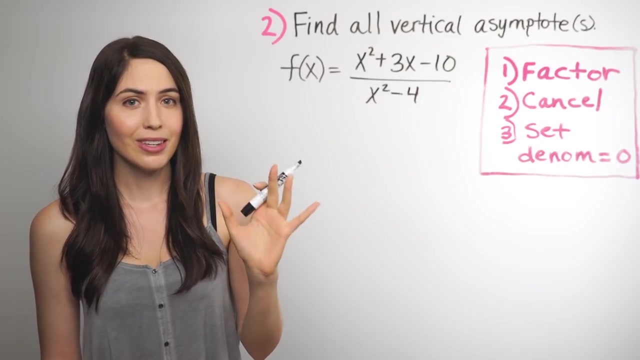 and now I want to show you a kind way to find the horizontal asymptote, so you can see it's a four-point line where factors do cancel. okay, so let's look at another one. say you need to find all the vertical asymptotes of this another rational function. it's the same. three steps to 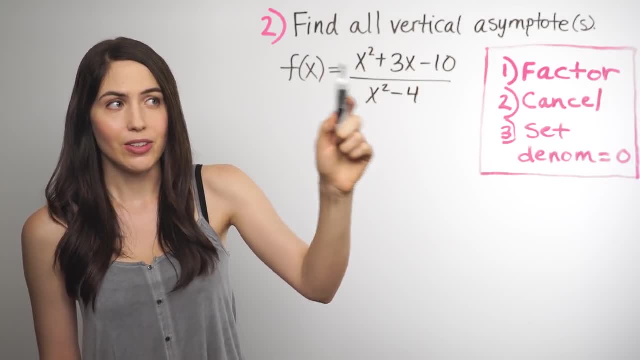 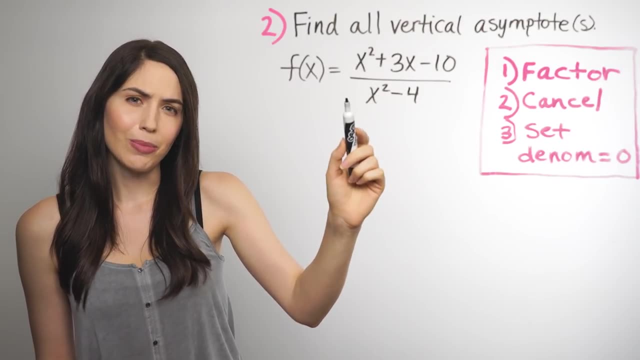 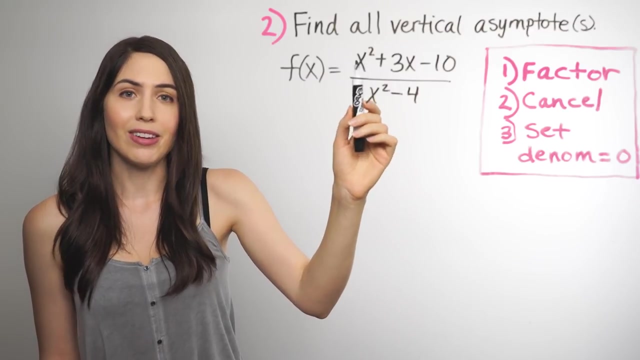 keep in mind. so first try to factor as much as you can. if you try to factor the top, this is a quadratic that you can break into two factors. when you do that, multiply to negative 10 and add to positive 3.. Those two numbers would be positive 5 and negative 2,. 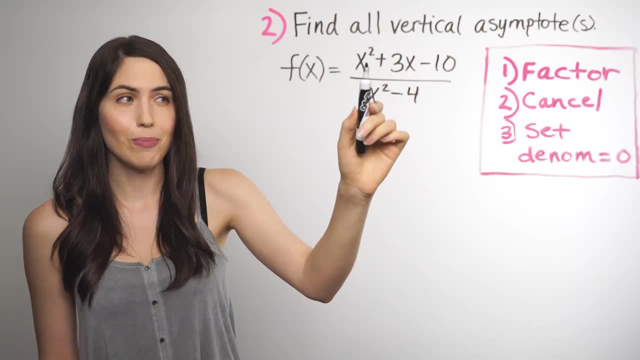 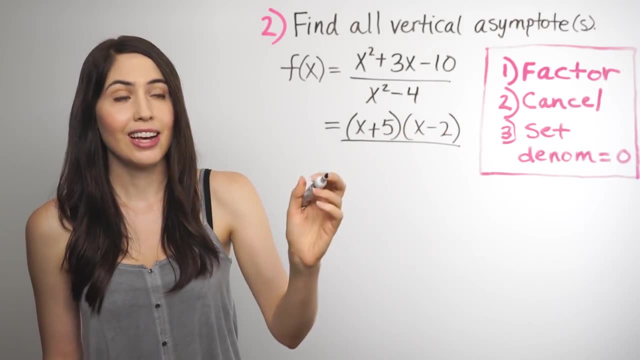 since 5 times negative 2 is negative 10, and 5 plus negative 2 is positive 3.. And now see if you can also factor the denominator x squared minus 4.. I know that this looks different from the top. 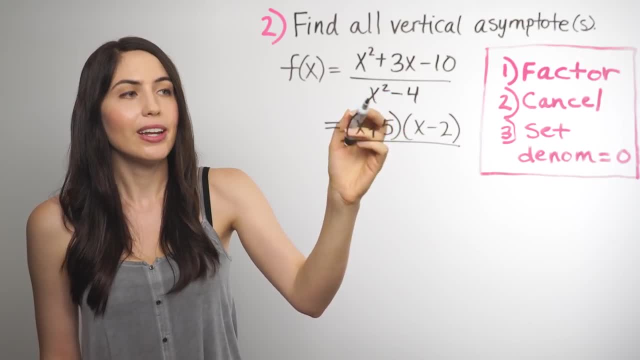 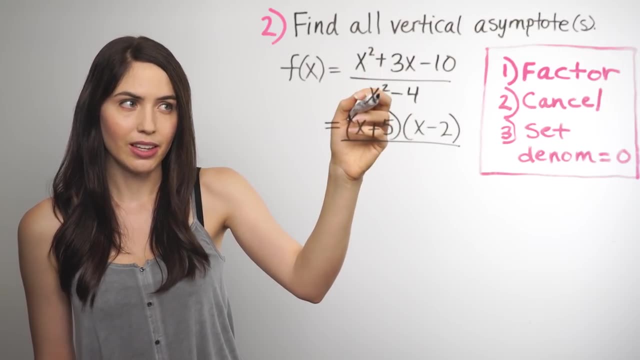 it's not a trinomial, there's no middle x term, but it is a difference of squares. 4 is a perfect square, so it fits into the difference of squares formula. So you can break this into two factors that start with x. 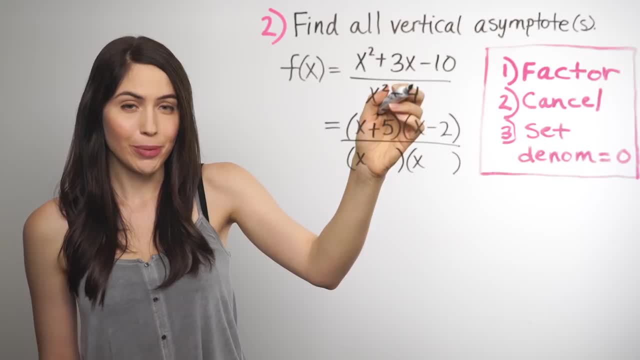 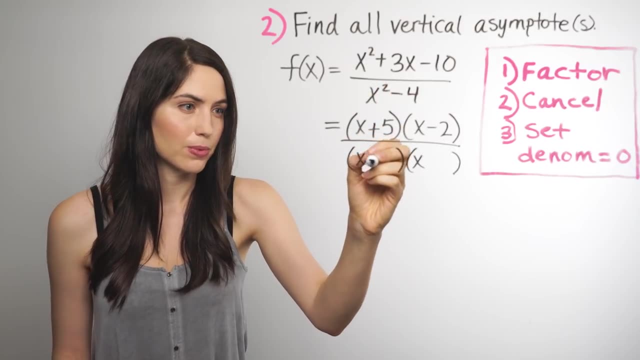 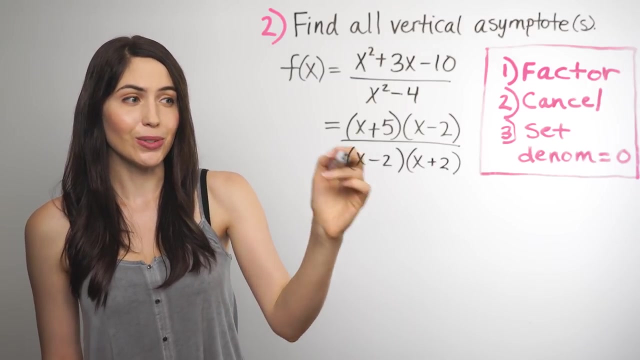 And using the difference of squares formula, since 4 is a perfect square, that's 2 squared. this breaks into x plus 2 times x minus 2.. And if that is an issue for you, feel free to look that up- the difference of squares. but you can also check this. 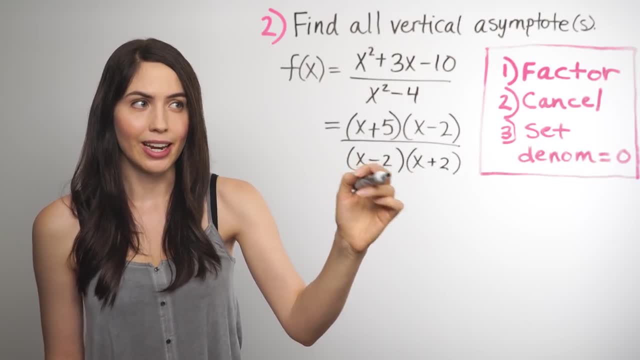 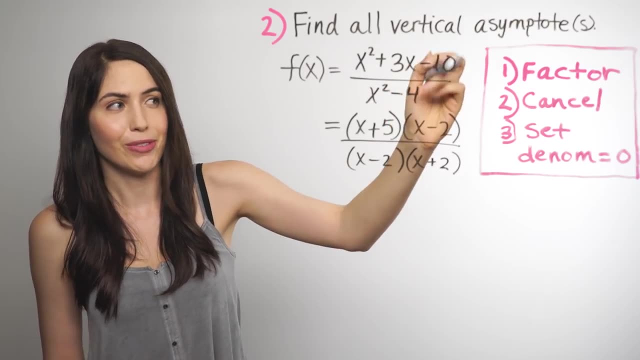 if you've multiplied this out and foiled this out, you would end up getting this back, so that works. Anyway, you've factored the top and bottom as much as possible. so that was the first step. Second step is see if there's anything the same on top. 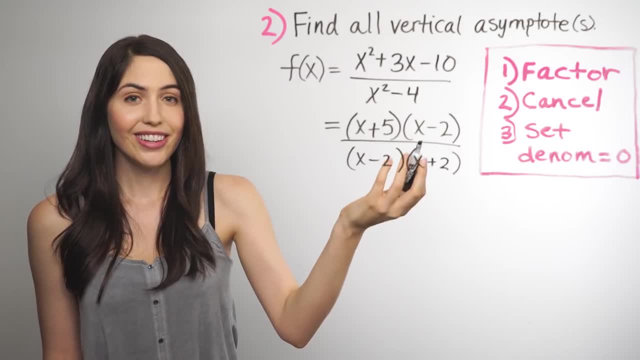 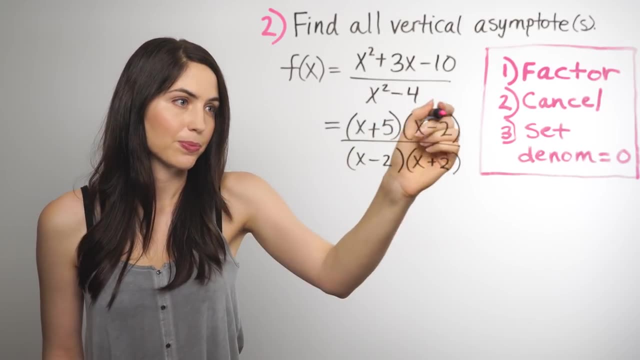 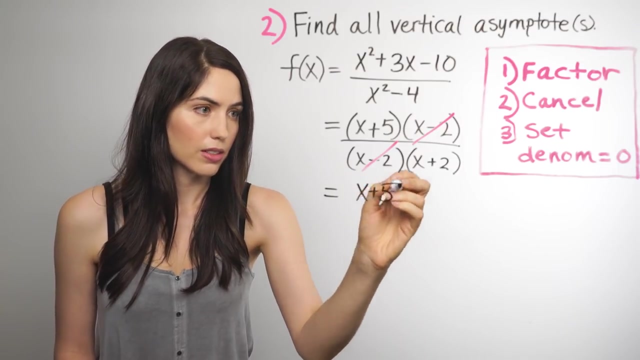 and bottom that you can just get rid of, just cancel. Here there is the x minus 2 is on top and bottom, so we can get rid of it. Simplify by cancelling it out and write what's left, And only after simplifying like we did, 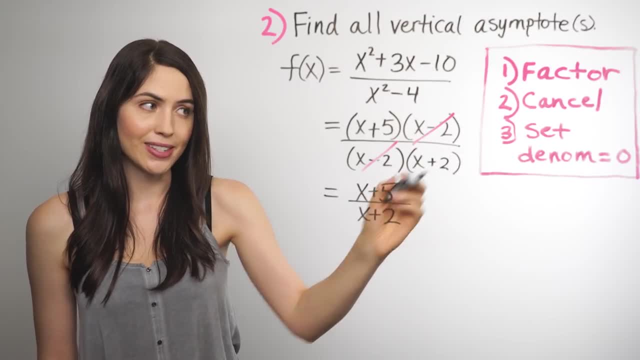 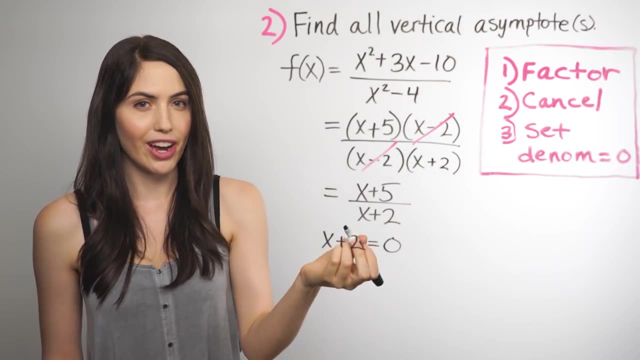 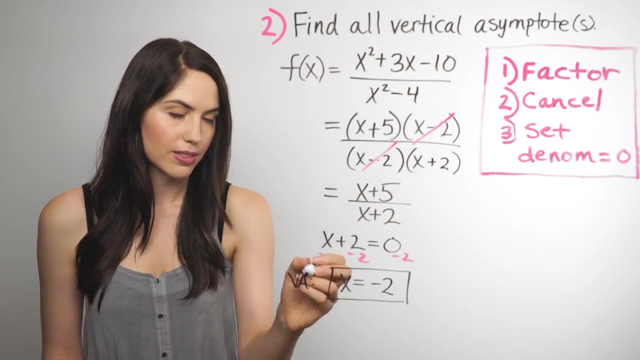 do you take the denominator and set it equal to 0.. That's the last step. take the bottom, set it equal to 0.. Solve for x, Which I'm sure you know how to do to solve for x and get it alone. 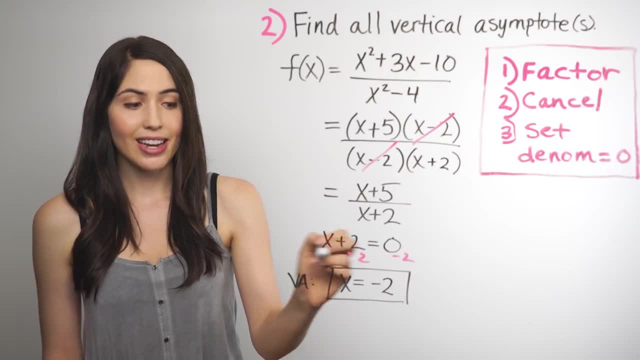 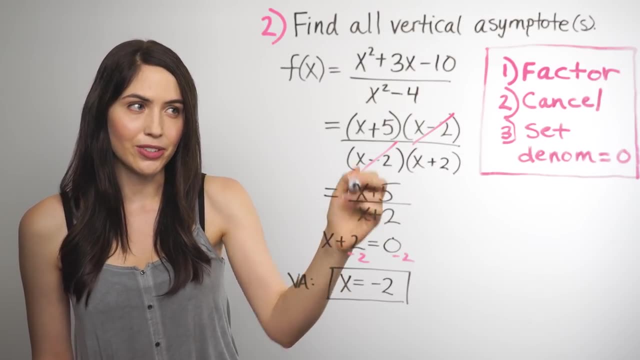 but when you do, you get x equals negative 2. And that is the vertical asymptote. you just have 1 this time. That's fine. it came from what was left in the denominator after simplifying like we did. Those cancelled terms those other ones did not end up giving us. 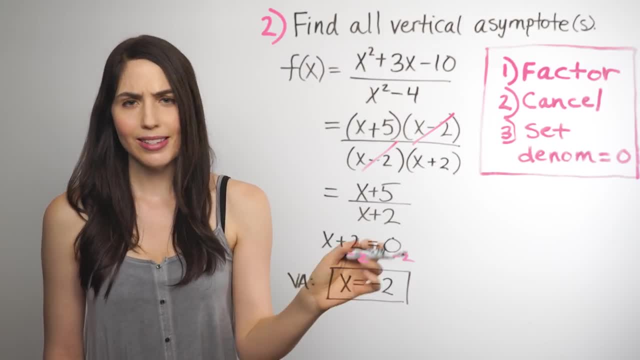 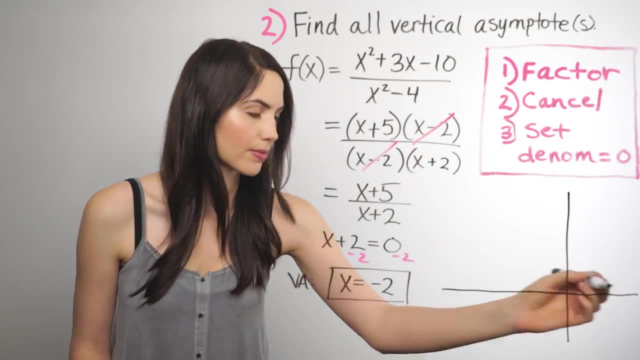 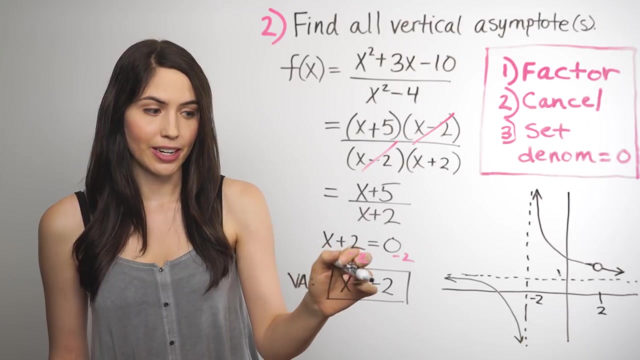 a vertical asymptote. So, by the way, what does this look like on a graph? and what happened to those cancelled terms? What was that about? Let me show you. Okay, so here's what this looks like. Your answer was just this: x equals negative, 2 for the vertical asymptote. 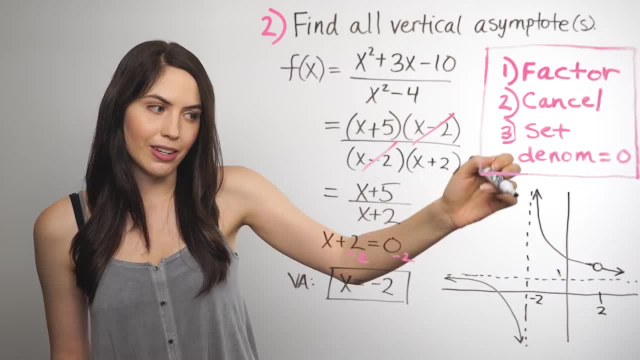 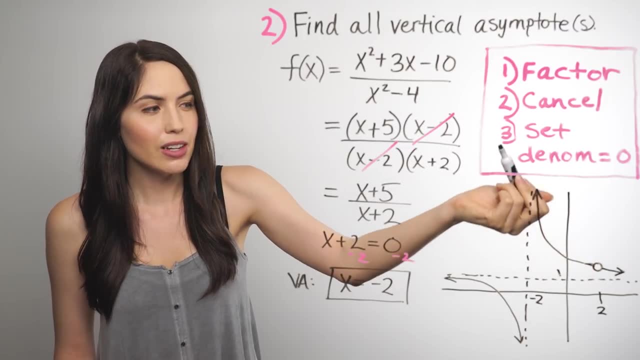 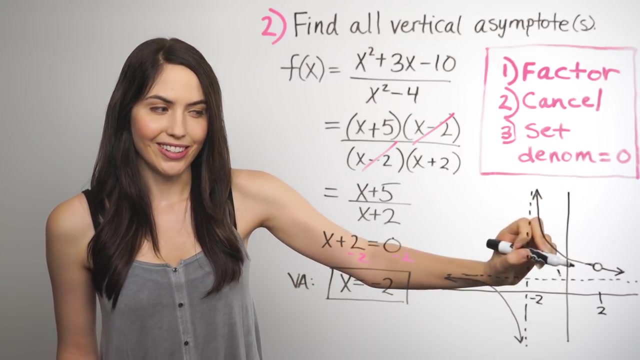 On the graph that corresponds to this dotted vertical line here and for the curve the graph, it will get very close to that dotted vertical line but never cross it or touch it. on this side and on this side, This other dotted vertical line. 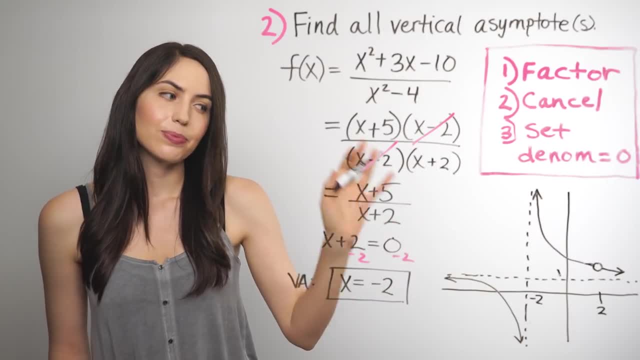 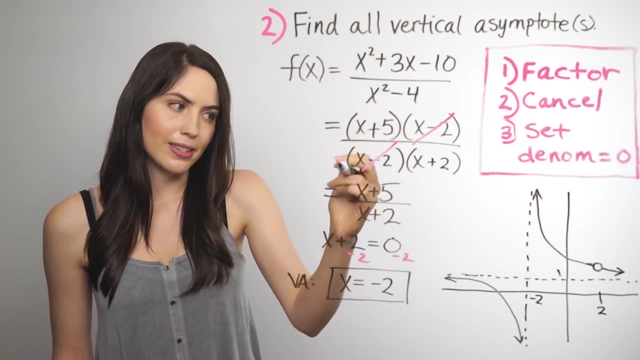 is a horizontal asymptote, and so that's another topic. But I want to show you what happened to those cancelled terms, just so you know. When that happens, it creates a hole in the graph of removable discontinuity, because at that point, at x equals 2,. 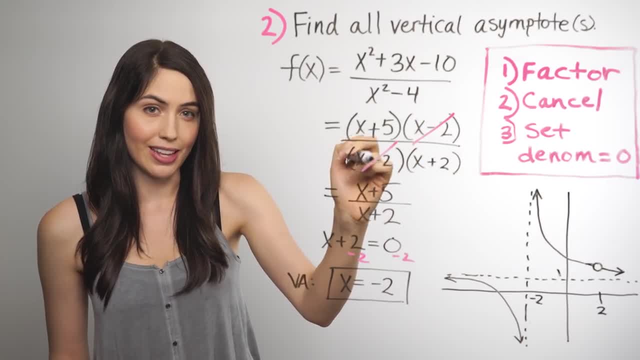 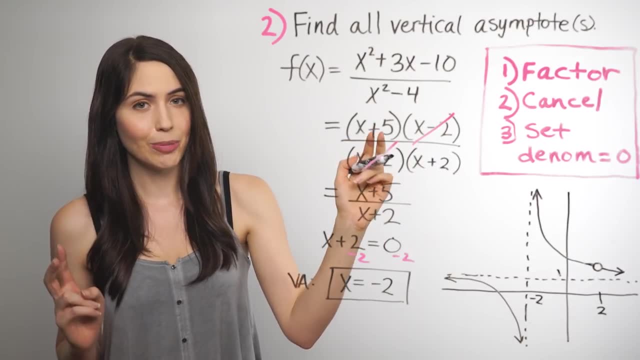 it made this equal 0 and this equal 0, and whenever you get a 0 over 0 form, any time, it is indeterminate as to the value. 0 over 0,, by the way, does not equal 1.. 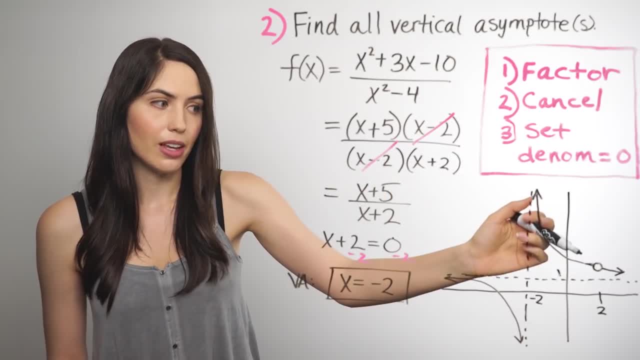 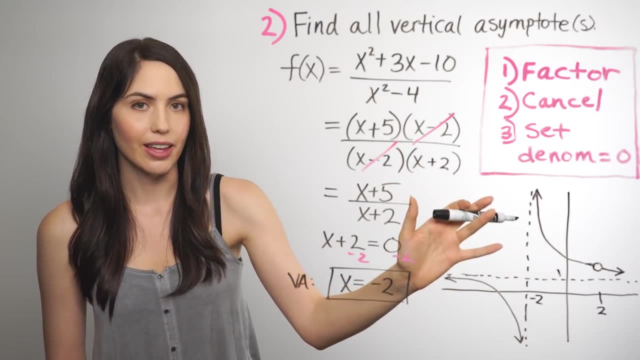 Does not. It's a special indeterminate form and it will be this gap in your graph if you zoomed in close enough. So that's just good to know. if you have to graph the whole thing, It doesn't matter, for just answering. 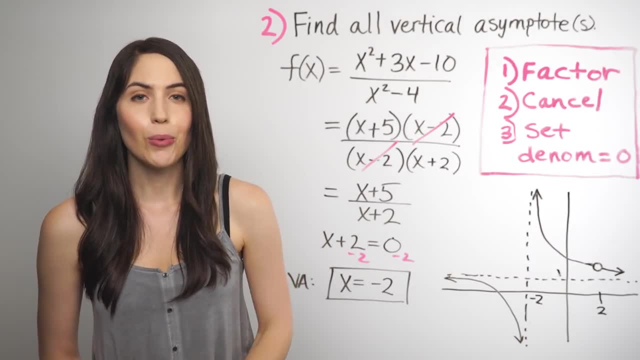 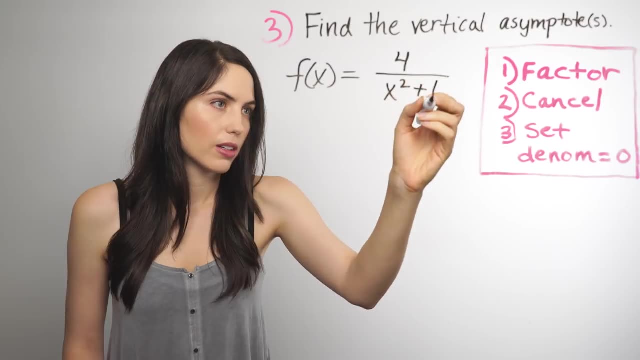 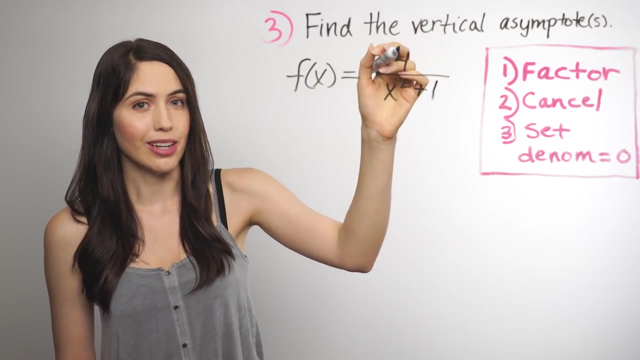 what the vertical asymptote is. Now I'm going to show you one last kind of vertical asymptote problem. Okay, here's one last kind. This kind looks much simpler than the ones before. It just has a number on top, just a constant. 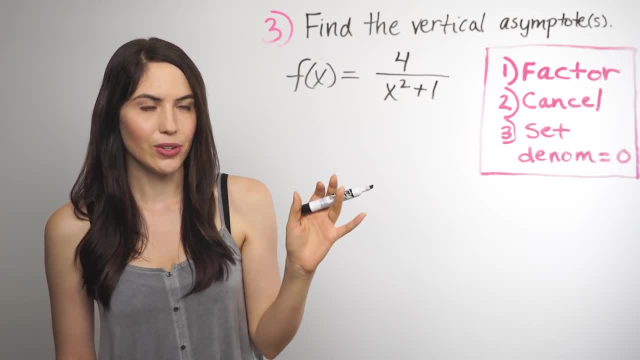 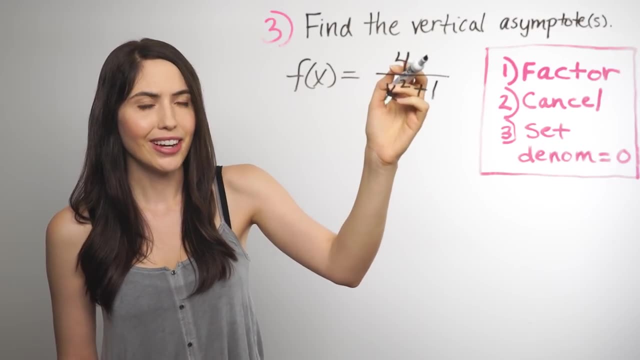 But that could throw you off that. it's so simple. So I want to show this to you. Still, try the same three steps. so try to factor the top and bottom. Can't factor the top, it's just a number. Try to factor the bottom: x squared plus 1.. 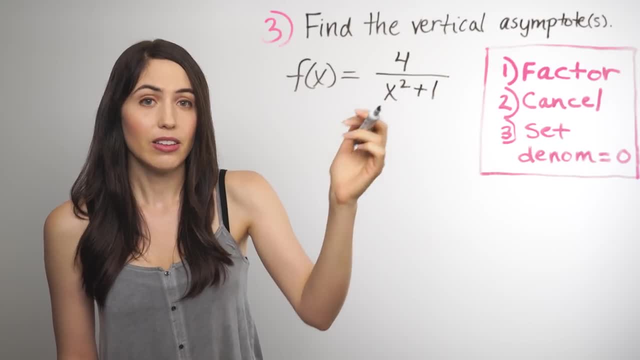 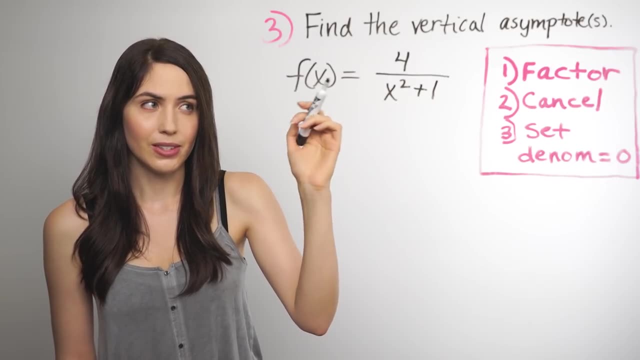 Turns out you cannot factor that If it had been x squared minus 1, you could use the difference of squares to factor using the difference of squares, formula x plus 1, x minus 1.. But since this is a sum of squares, 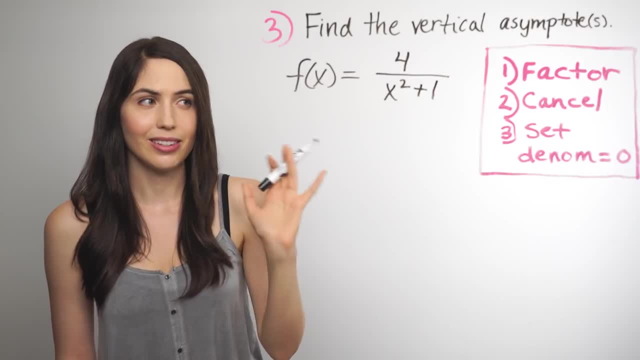 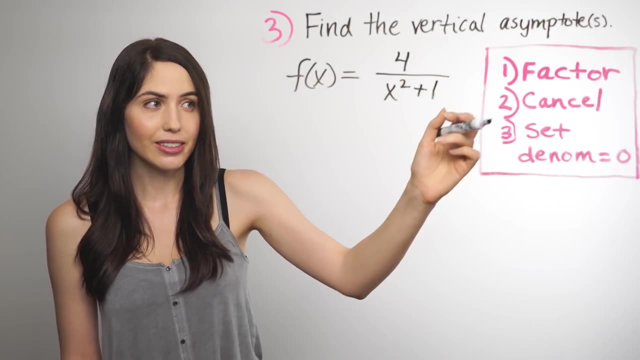 x squared plus 1 can't factor. Go ahead and try. It's not factorable, So move on. There's nothing you can cancel either. So really, if you can't factor, anything can't cancel. just take the bottom and set it equal to 0.. 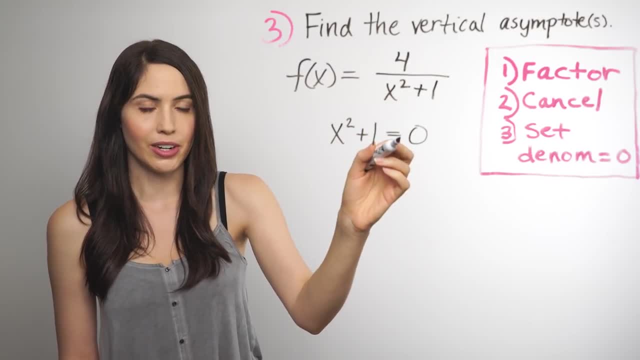 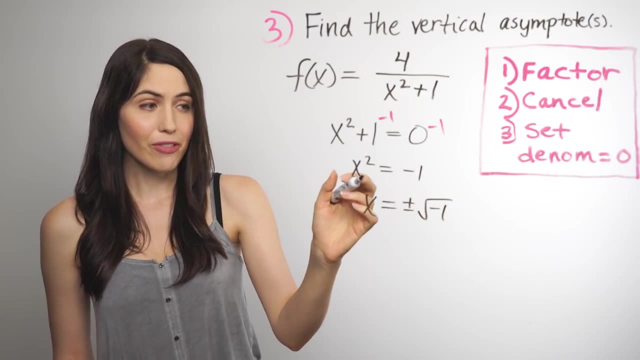 So take the denominator x squared plus 1,, set it equal to 0, and solve for x. Okay, when you try to solve for x, you get x squared equals negative 1, and at this point to get just x alone. 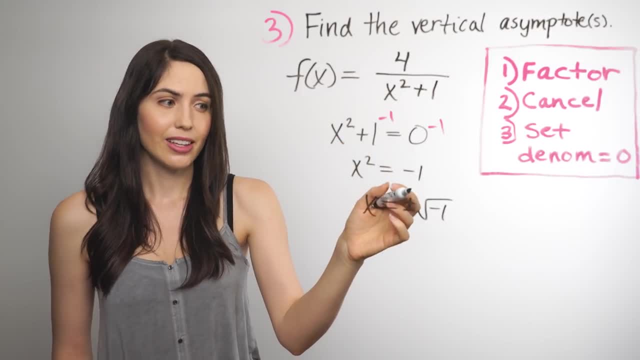 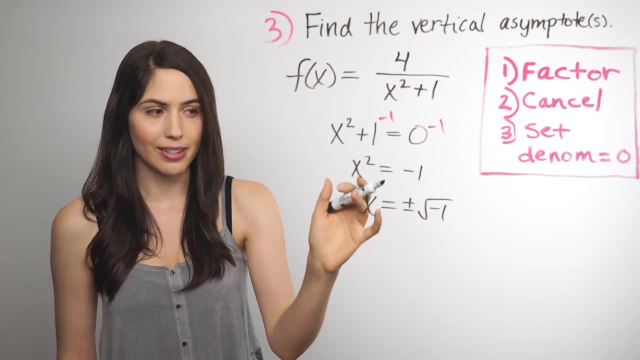 typically you'll, just you would square root both sides. Here you get plus and minus the square root of negative 1. That is imaginary, complex number and this means that you get no vertical asymptote If you get no real asymptote.